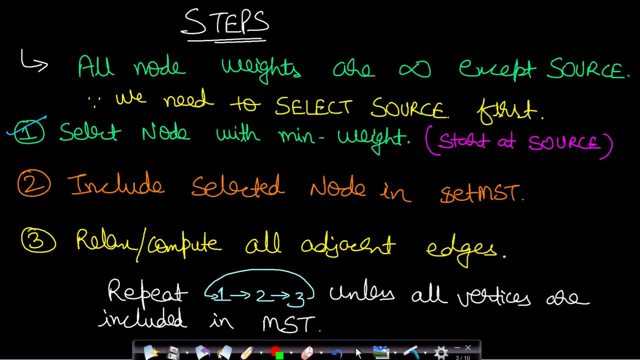 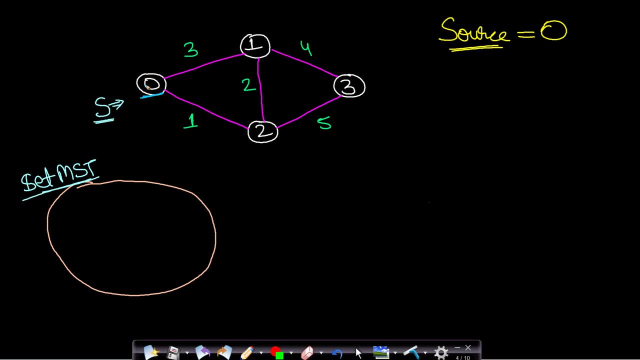 where will you? how will you find the minimum weight? so let us assume that this is your given graph, okay, and let us assume that you will be starting at this node zero. so how will you select which node to start and where to start start, and how will you select about the node weights? so what we will do is, since this is the 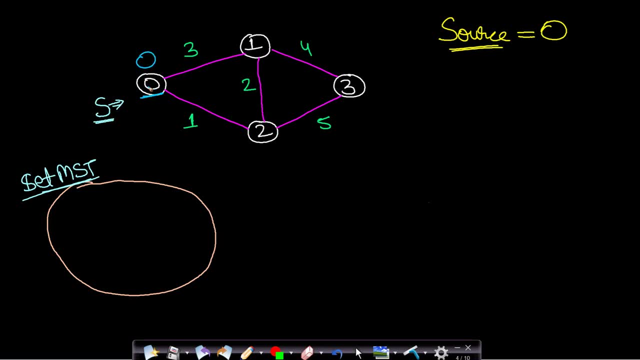 starting node. we will assign value 0, that is, weight 0 here, and all the other weights will be assigned as infinity. and why have we done this? because we want this source node to get selected first and since our selection criteria involves the minimum node, weight to get selected first. 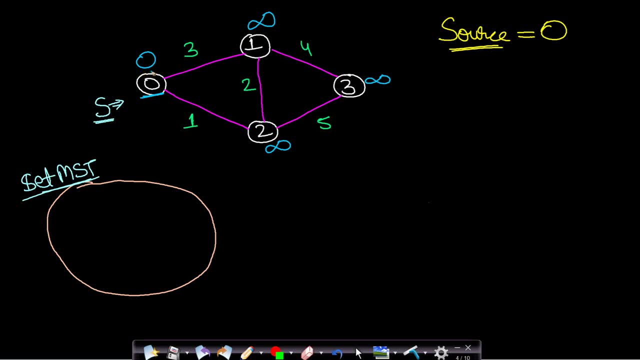 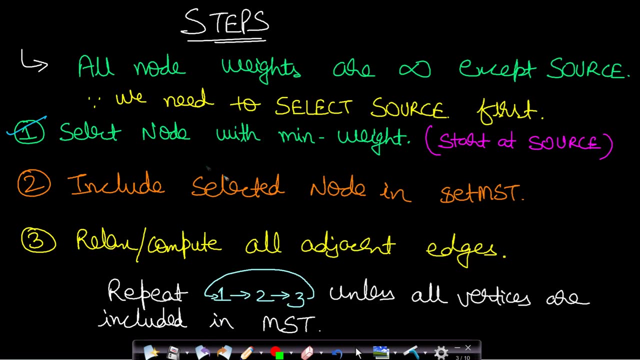 therefore, the source node will always have the minimum value, which is 0, and rest other nodes will be having value infinity, so that they don't get picked okay. so this is the logic behind this first step: select the node with minimum weight, so all the node weights are infinity initially. 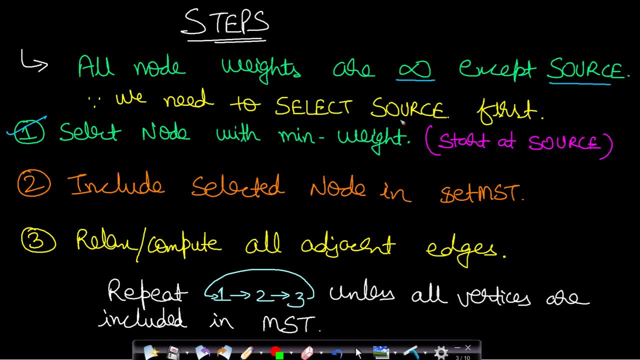 except the source node, since we need to select the source node first. okay, so this is the logic behind our initial setup. so, after doing the initial setup, we will be doing this step one, where we will be selecting the node with minimum weight, that is, we will be starting at the source. 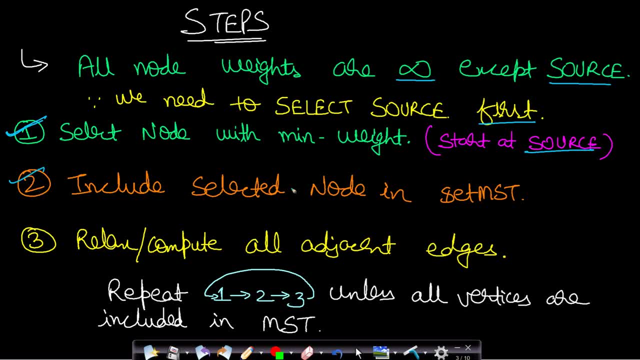 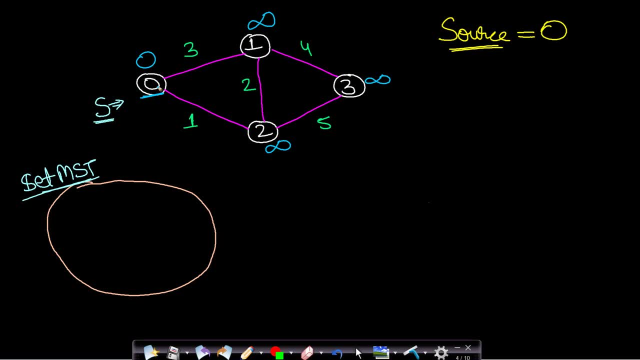 node you now. the second step is to include the selected node in our MST set. so what is our MST set actually? whatever node is already processed that we will not process it again, so that duplicate nodes will get avoided. so how it is done, let me explain you okay. in the first step, this 0 will get selected. 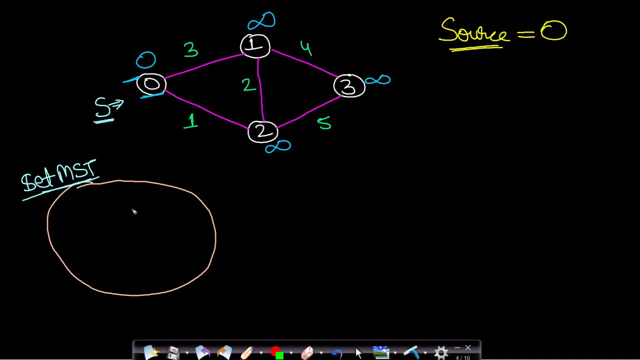 because this is having the minimum value. so this will be processed, and so let me also draw the minimum spanning tree. this will be the minimum spanning tree. okay, now, since this 0 has been processed, we need to keep track of all the processed nodes, so this will be. 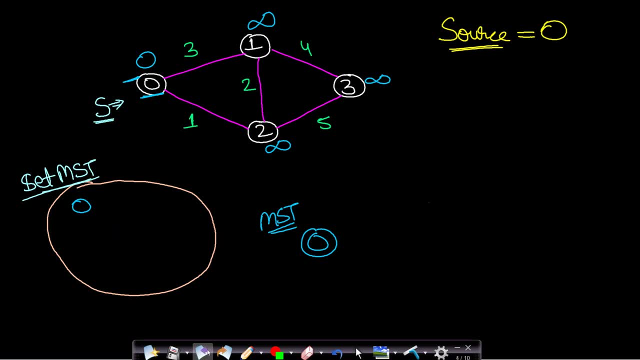 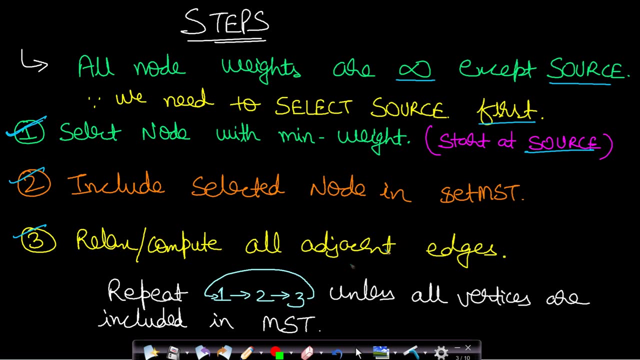 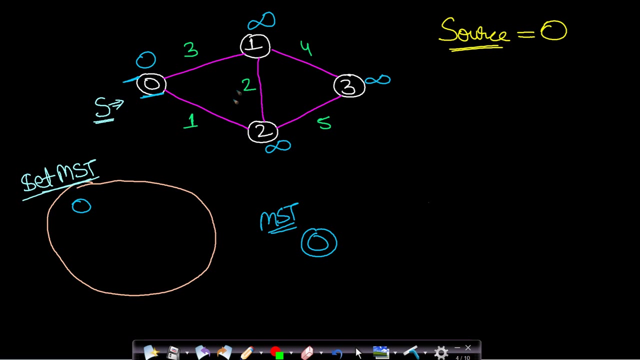 included in this set MST and after including this node in set MST, we will start with this third step. so third step says that relax or compute all the adjacent edges. so the adjacent edge of this 0, that is, the adjacent vertex of 0, is 1 and 2. so we will have to update the weights for 1 and 2. they are: 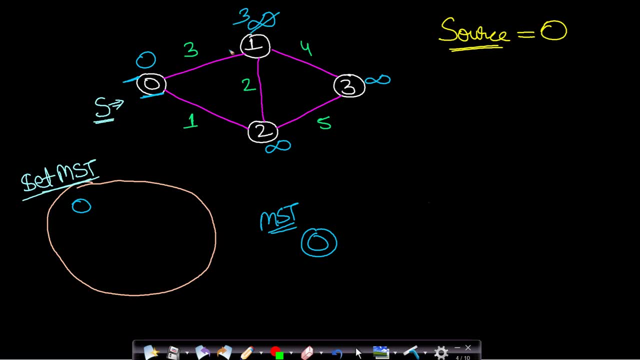 infinity, so this will now be 3, since the cost of 0 to 1 is 3. now the cost of 0 to 2 is infinity, so this will be 1. okay, because 1 is less than infinity, so whenever the value is lower, it will get updated. 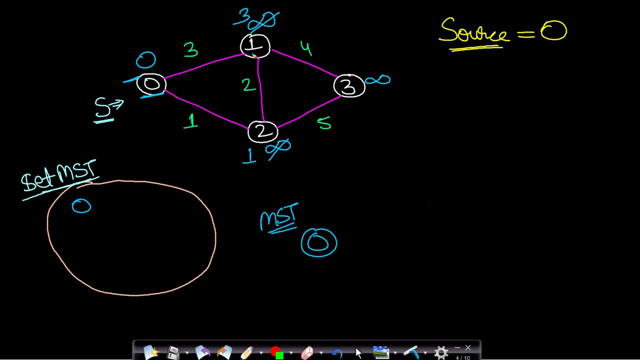 now, the adjacent values have now been updated. so what is the next step? the next step is to select the minimum values among these vertices. so we will have to update the weights for 1 and 2. so this is alkver 3. i have like this one, so we have 2 and 3. we want to filter it here, so we have 4 vertices. 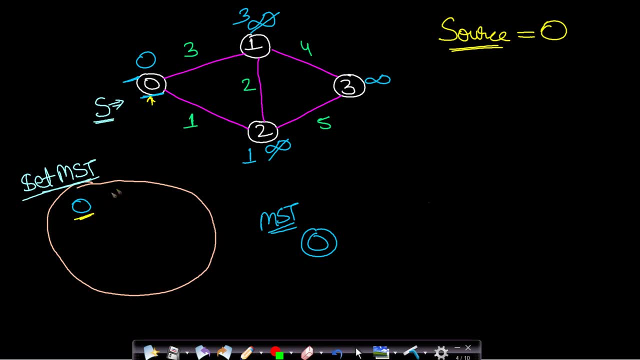 so we will start comparing from this. node zero, so not 0, is having value 0. but this is already processed, as you can see that it is already present in set MST. so we cannot pick an already processed node. so we will check for this node one. node one is having value 3. node 2 is having value. 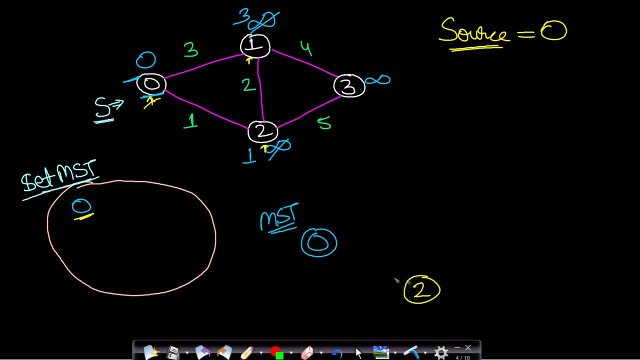 1, so it is better to select this node two. okay, mst. so 2 will be added to set mst. now we will relax all the adjacent edges or the vertices. so from 2 this 0 is the adjacent vertex, but this is already present in our set mst, so nothing will. 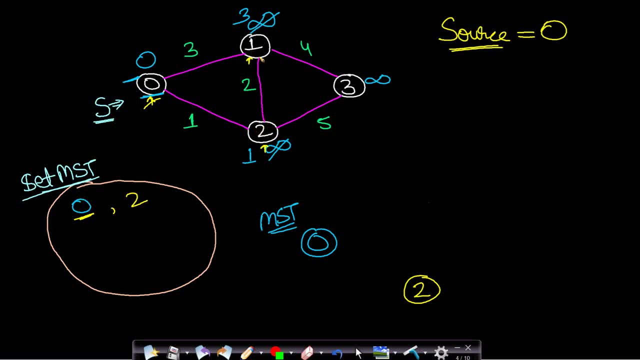 be done from this: 2- 1 is adjacent and the value at 1 is 3, so the new value edge weight is actually from 2 to 1. it is 2, so this will now get updated to value 2. okay, since 2 is less than 3 now from. 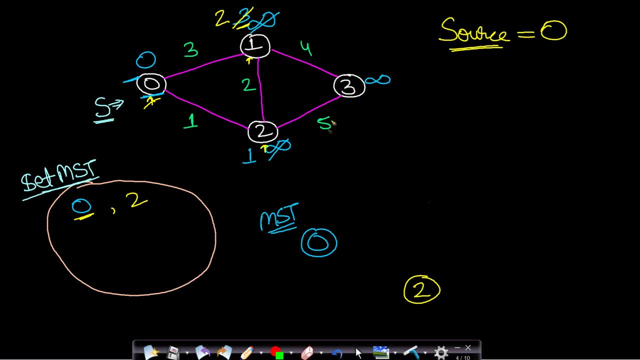 2. this 3 is adjacent, so from 2 to 3 the distance is 5 and the already stored distance is infinity, so 5 is lower. therefore, 5 will be stored here. okay, so all the adjacent edges have now been relaxed. so what is the next step? well, 0 and 2 have already been added to set mst, so we will again. 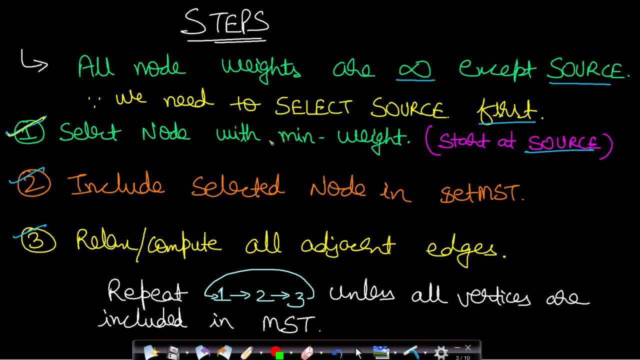 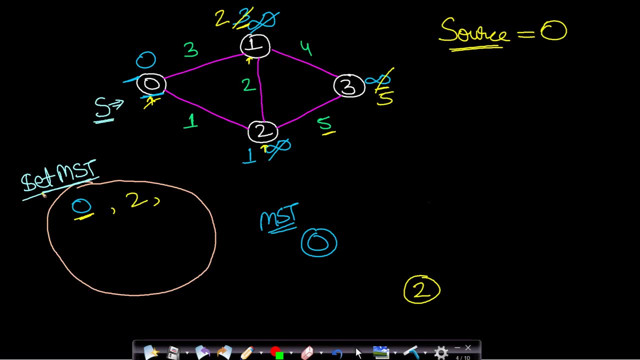 go back to this step 1. step 1 is to select the node with minimum weight. so we are left with just node 1 and node 3. these are already included in set mst, so we will start comparing from this. 0. 0 is already included in set mst, so 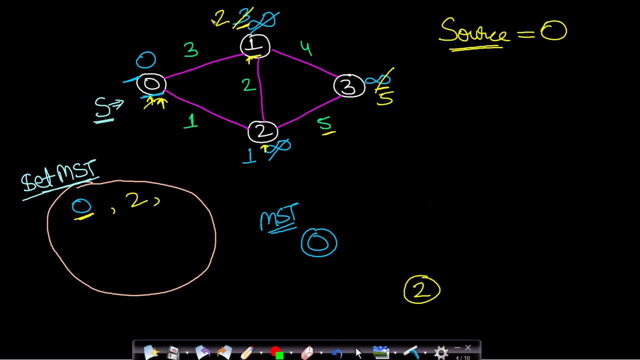 nothing will be done. this 1 is not included, so its weight is 2. 2 is already included and 3 is not included. its weight is 5, so the minimum weight you can see is 2, which is for 1. so now 1 will get included and, by the way, when you added this 2, this edge will also get added. 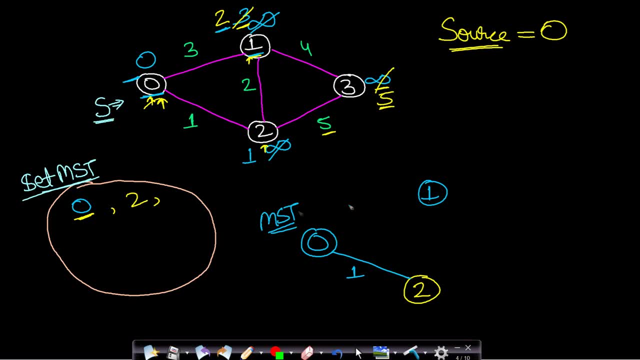 with weight 1. now this 1 will also get included. so 1 will be included in set mst as well. you will add this edge as well. weight will be 2, okay, and you will relax all the adjacent edges. so from 1 edge going to 0 will not be relaxed because 0 is already. 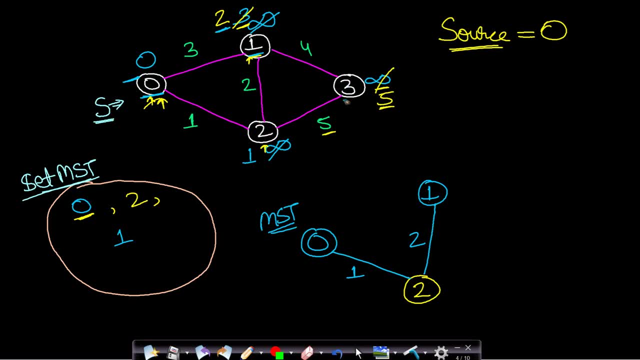 present in mst. 2 is also present in mst. 3 is not present in mst. so what will be the weight? the weight will be the edge weight from 1 to 3, which is 4. initially it is 5, so 5 is actually greater than 4, so it will get updated to 4.. 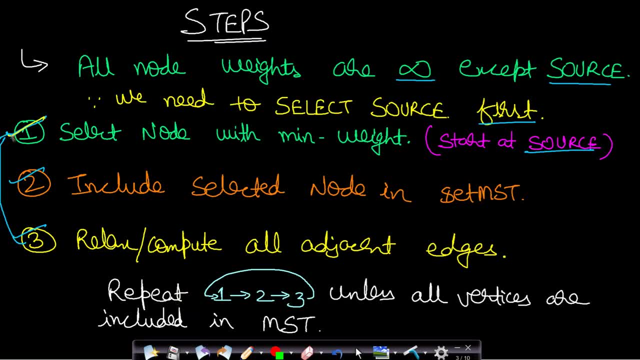 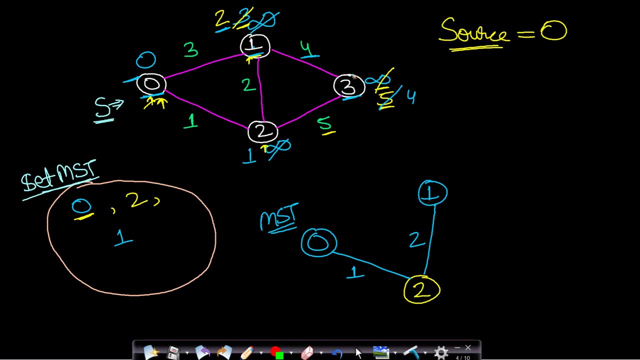 Now we will again go back from this step 3 to step 1, okay, and we will select the node with minimum weight. now the node with minimum weight is 3, because this is the only node which is left and this is having value 4, so 3 will get selected and 3 will be added to. 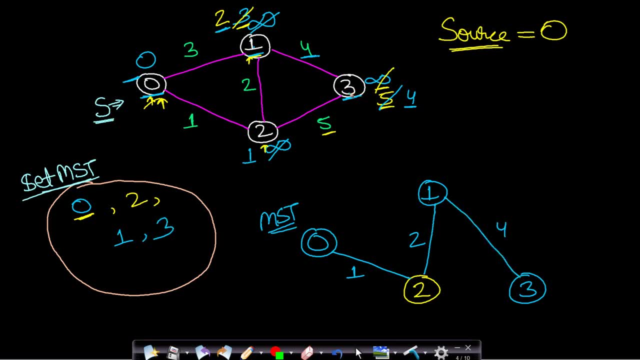 set mst and this edge will get added. now we will try to relax all the edges, but all the adjacent vertices have now been included. you can see that all the vertices of this entire graph are included in this set mst. So now we will start. 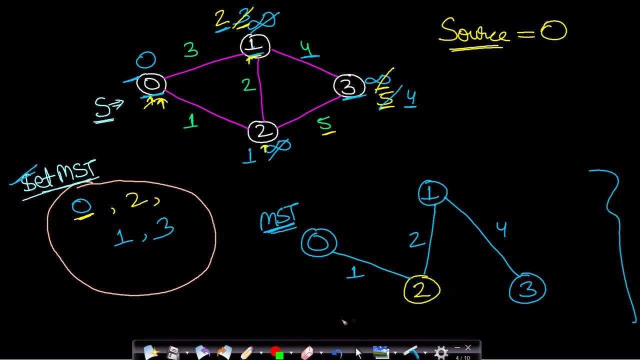 And whatever graph is formed, this is the resultant graph. so this will be our minimum cost spanning tree and you can see that in order to cover all the vertices, the minimum cost would have been: if you start from 0, then you go to 2 with cost 1. from 2, you go to 1 with cost 2. 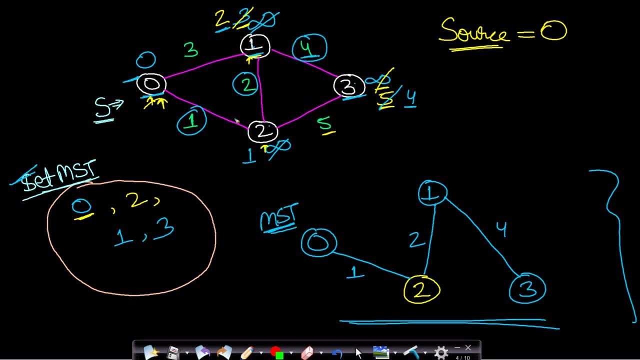 and from 1 you go to 3 with cost 4. so the minimum cost will be 1 plus 2 plus 4, which will be equals to 7. so using cost equals to 7, you can cover all the vertices of the given graph. so this is the minimum cost and this is the minimum cost spanning tree. so I hope. 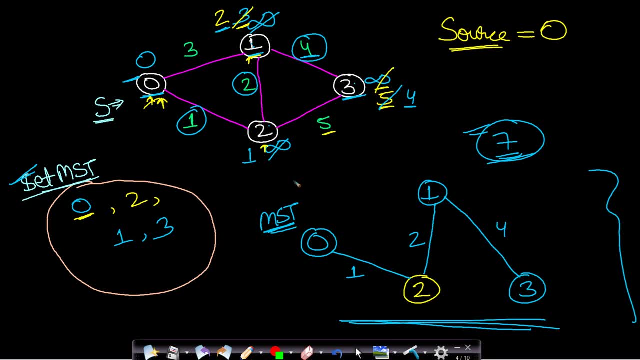 you understood. this is a very simple example, okay, so what can you observe here? you can observe that we started from this node 0 and we are expanding only at the adjacent nodes, that is, wherever the mst is starting. we are expanding only adjacently. okay, we are not. 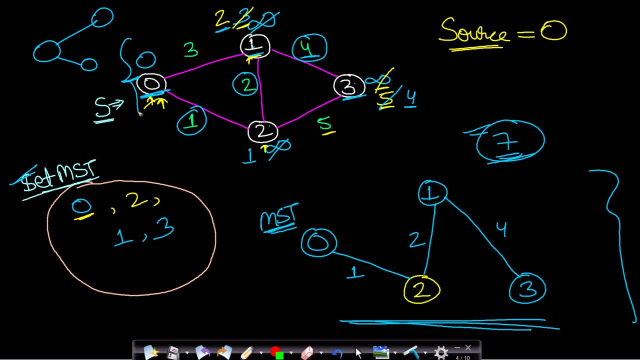 expanding randomly. so in this case, for prim's algorithm, the expansion only happens at the adjacent node. but for Kruskal's algorithm I will be explaining you in the next video. there we will be expanding randomly. okay, so from 0, where will we grow? we will have to. 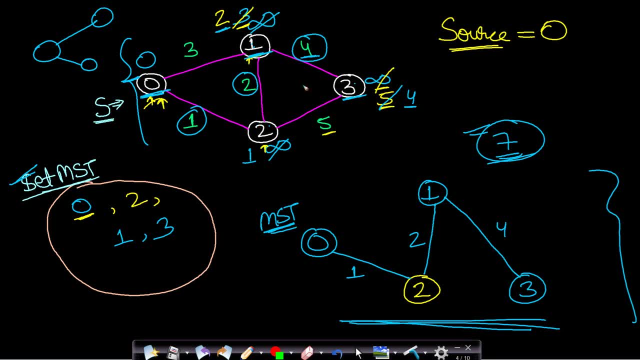 select either of this, node 1 or node 2. we cannot go from 0 to 3 because the algorithm is designed in such a manner that this will be 0 and rest. all nodes will be having value infinity. so we are relaxing only the adjacent vertices. okay, so when we relax the adjacent 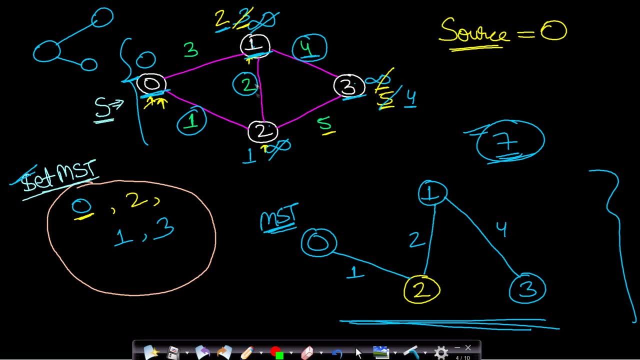 vertices, we will be having, of course, the minimum values, and so every time we do the first step for selecting the minimum weight for a vertex, always the adjacent node will get selected. okay, so this is the reason why we are expanding adjacently and not randomly. so this is also 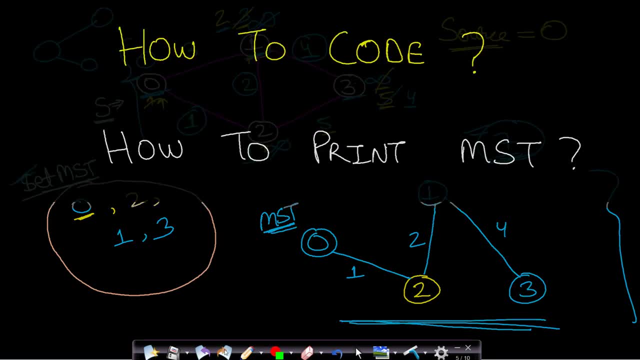 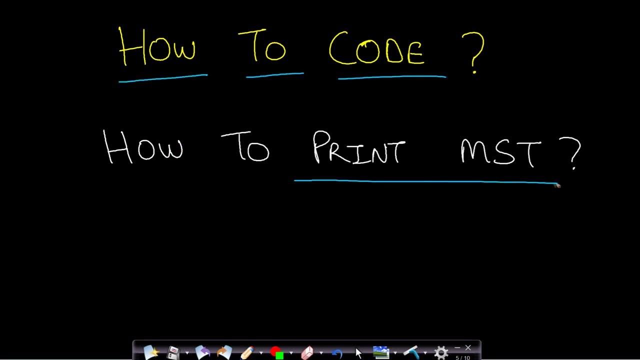 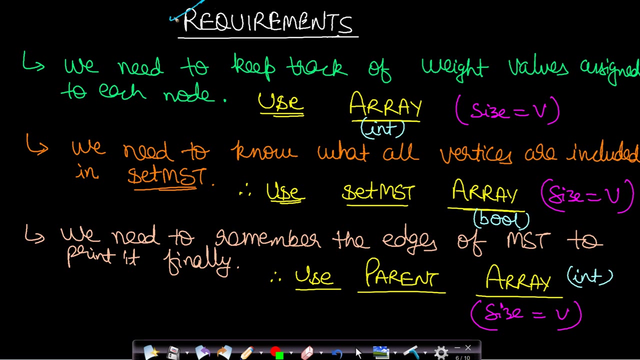 an important observation. but having understood the algorithm, the theory part is very easy. now you might be wondering how to code this algorithm and how to print the mst. well, we will be explaining these two things in the next part. so first we will be analyzing. 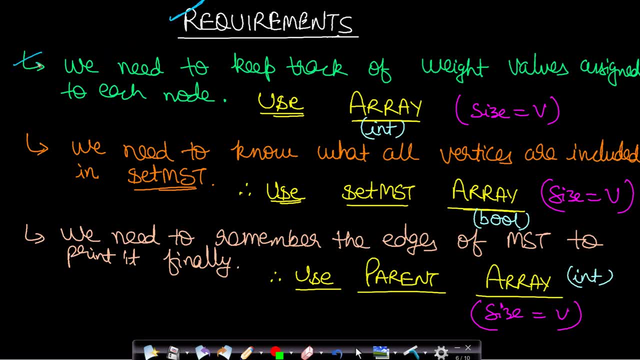 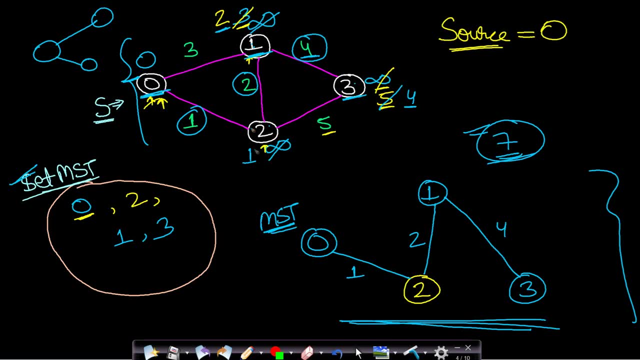 what are the requirements in order to code? so our first requirement is that we need to keep track of weight values assigned to each node. so, as I have already said that in for these four nodes, initially we were assigning infinity, for 1, 2 and 3 and for 0 we were assigning 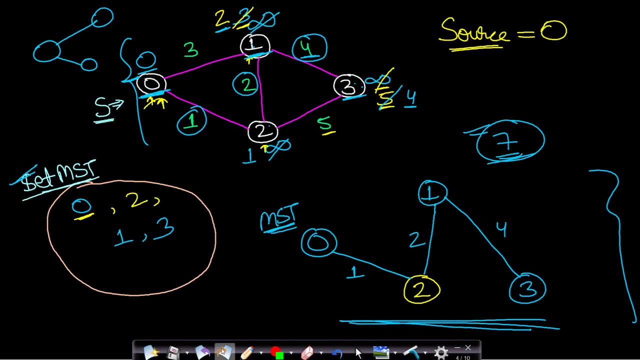 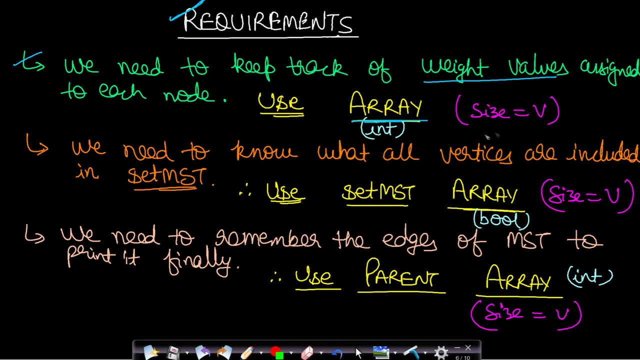 0, so we need to keep track of all these values. so, in order to keep track of these values, we will be using an integer array. and what will be the size? the size will be equals to the number of vertices. okay, because we will be storing the weight for the vertices only. I hope you understood this requirement. 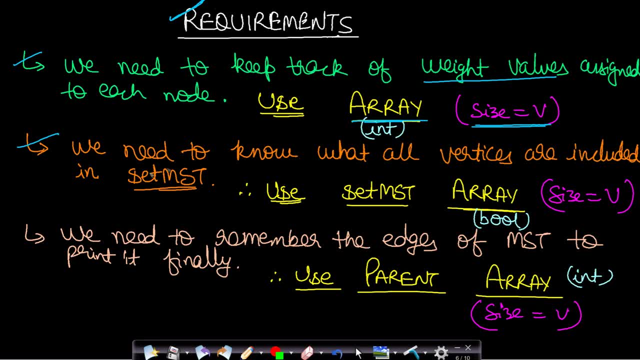 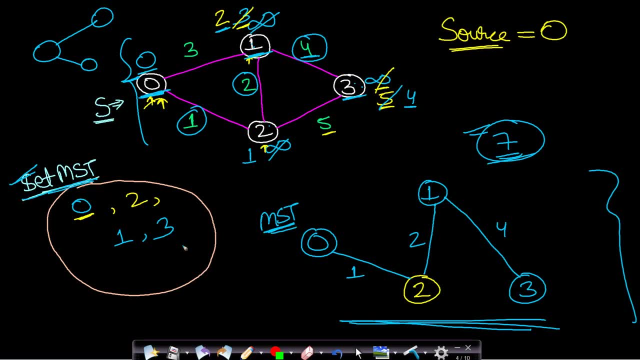 now, the second requirement is that we need to know what all vertices are included in our set, mst. so we were required to maintain a set, which will be the mst set, which will keep track of what all nodes have already been included in our mst, so that no duplicate. 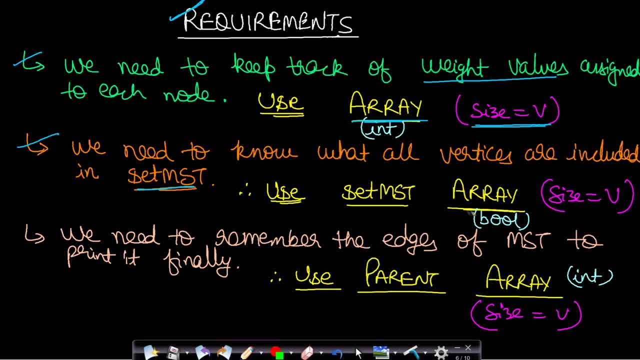 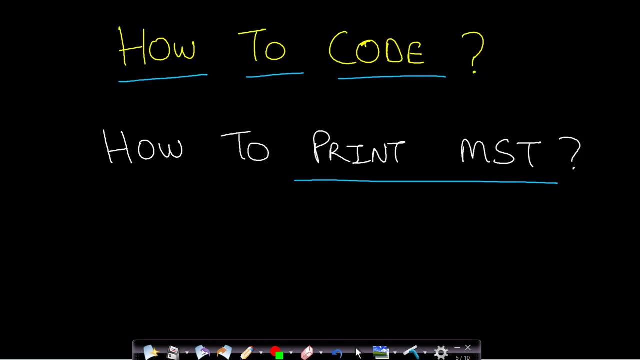 nodes get included. so for that, we can do that, we can use a boolean type array, and the size will be equals to the number of vertices. okay, now the third requirement is that we need to remember the edges of the mst in order to print it. finally, and so in order to remember these edges, that means from 0 to 2, 2 to 1, and. 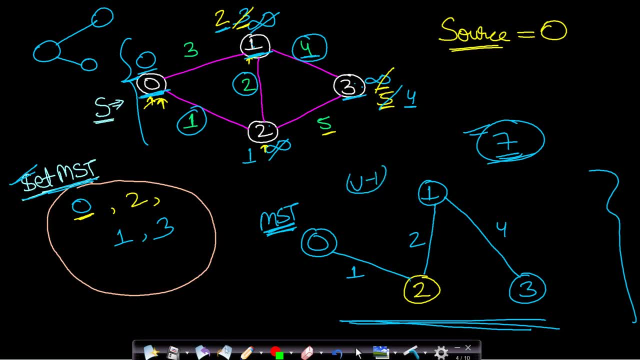 1 to 3. we need to remember these v minus 1, number of edges. so, in order to remember those edges, what we can do is we can maintain a parent relationship. in this case, you can see that parent of 2 is 0, parent of 1 is 2, parent of 3 is 1. if we can remember like this, then 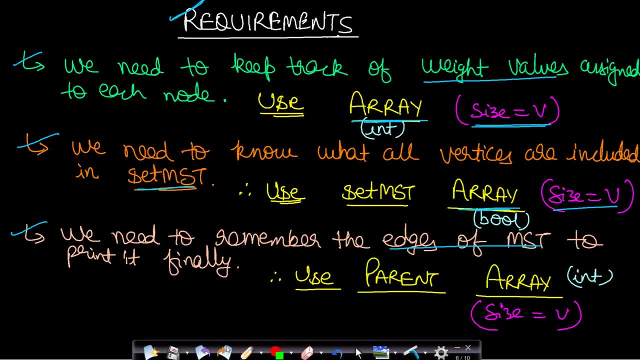 we can simply print this mst. therefore, in order to maintain this parent relationship, I will be using a parent array. so this is a very simple logic to understand. so if you do not understand this part, then you should watch my brute force disjoint set video at the link will be present in the description below. now the size for this will be. size is: 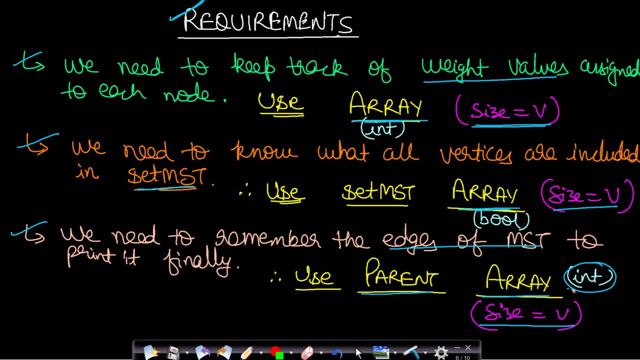 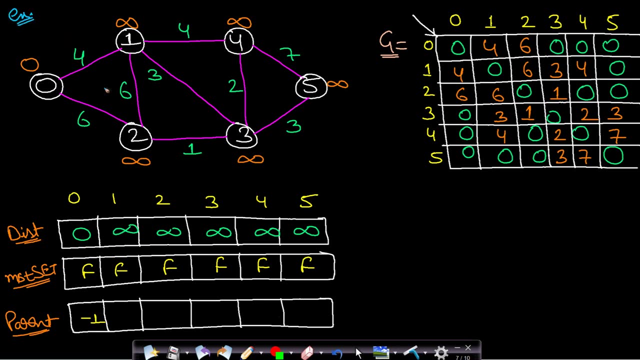 equals to number of vertices, number of vertices, and this will be of integer type. so I hope you understood all these three requirements, and all for all these three cases, we will require arrays. so this will be a very simple implementation. now let me first explain you an example, and after that we will look. 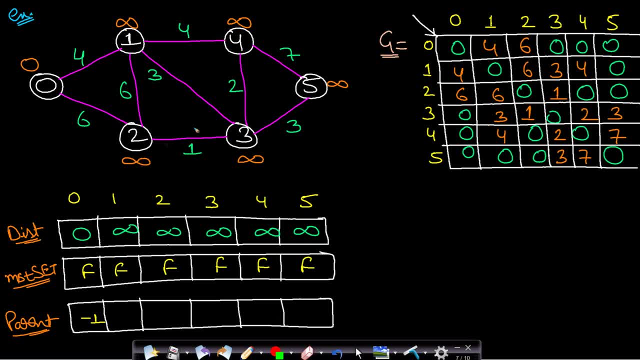 at the code. so first you will be presented with the graph. now, in what way you can represent the graph? you can either use an adjacency list or an adjacency matrix. so in this case I will be using an adjacency matrix for simpler explanation. okay, so this is the given graph and we will be given actually. 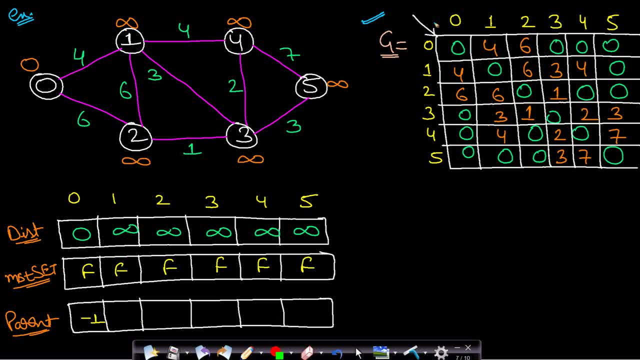 this adjacency matrix or we can form it now. once we have found this adjacency matrix, and since this is an undirected graph, these values in the upper diagonal and lower diagonal will be symmetric. that means the corresponding position values will be same. they will be symmetric about this top diagonal, that is, top left diagonal. okay, now, once you have this, 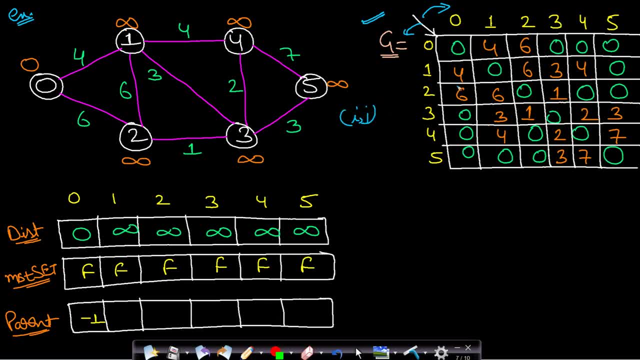 matrix I comma J. value of the matrix indicates that, in order to go from node I to node J, what is the edge weight? okay, so let us see this value. in order to go from this node 2 to node 3, what will be the weight? the weight will be equals to matrix at 2, 3, which will be 1. so in the graph, 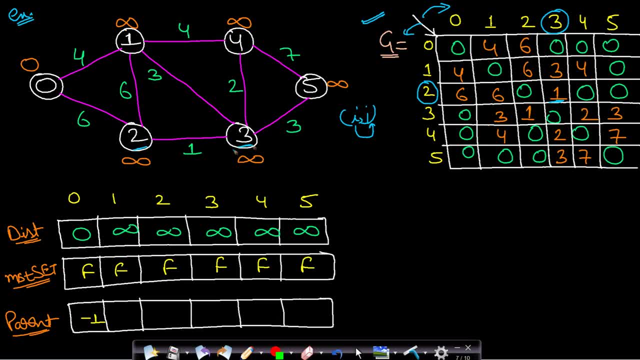 you can see that if you want to go from 2 to 3, then the edge weight is 1. so I hope you understood this logic as well. now, once you are given this adjacency matrix and you have maintained three different arrays for our three requirements, as I have already explained, 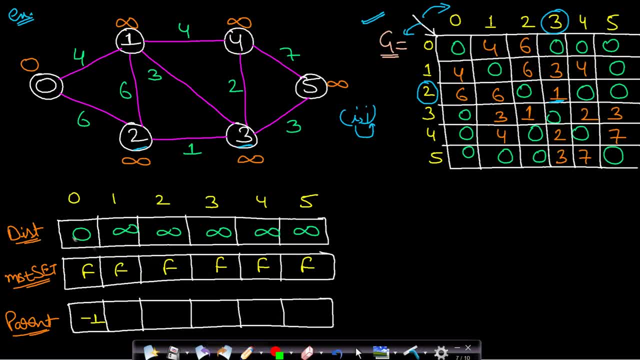 you, then we can start the algorithm. now let me just explain you the initial values of all these three arrays. so first one will be the distance array, and for that I have already explained that only the source value will be zero and all other values will be infinity. 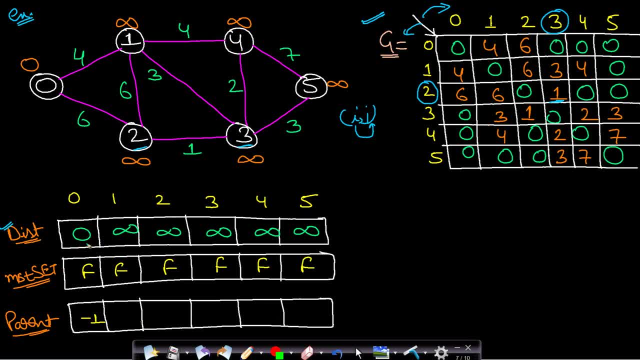 because the first step is to include the node having minimum weight, so that this source node gets selected first. We will make it zero and other nodes as infinity I comma j. So this is the logic for this initial values of distance array. now we will also be having 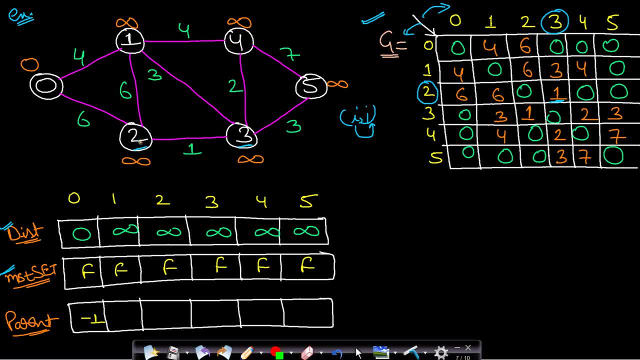 MST set, which will keep track of what all nodes are included in our MST. so initially, no node is included in MST, and so all the values will be false. now we will also be having the parent array and this will keep track of the MST. that means what MST structure is. 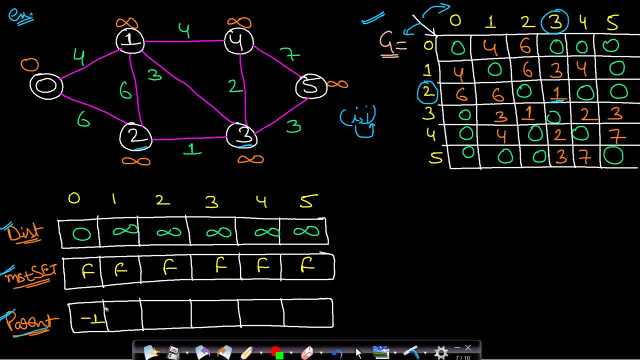 formed. so this will be valuable in printing the MST structure. now for this parent array for the source node, we will be having no parent, and we are assuming that source node is zero. so since source node is zero, it will be having no parent and so value will be minus. 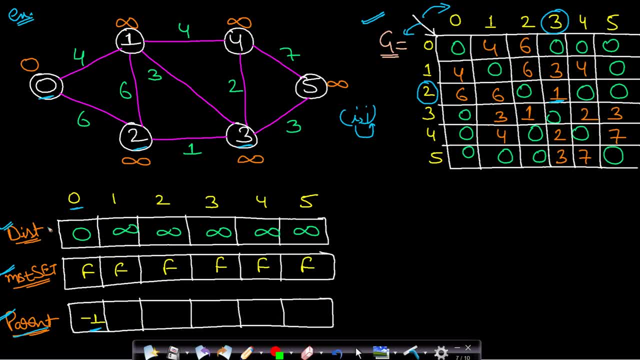 one rest, all values will be empty. okay, so these are the initial value explanations and I hope you understood this now let us start with the algorithm. now what we will do is we will start with this value, zero. so zero will be included in our MST. so the first step. 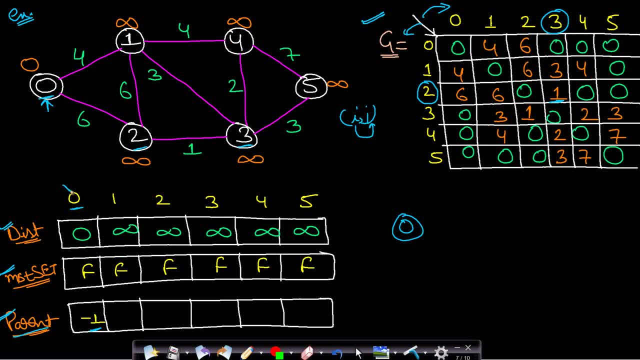 is to pick the minimum node value. So zero will be picked first. now, since zero is picked, we will make zero value as true, since this is included in our MST set. and now what we will do? we will relax the adjacent edges, so the adjacent edge is going to vertex one and vertex two, so vertex one is having 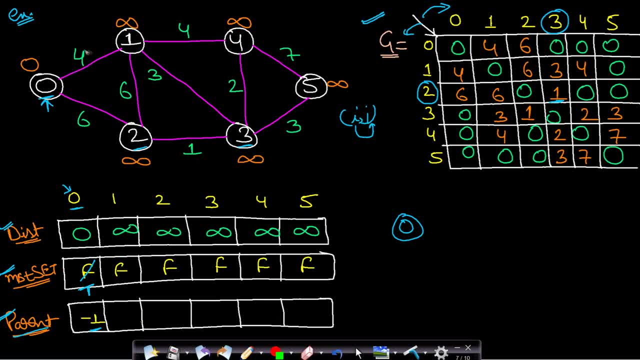 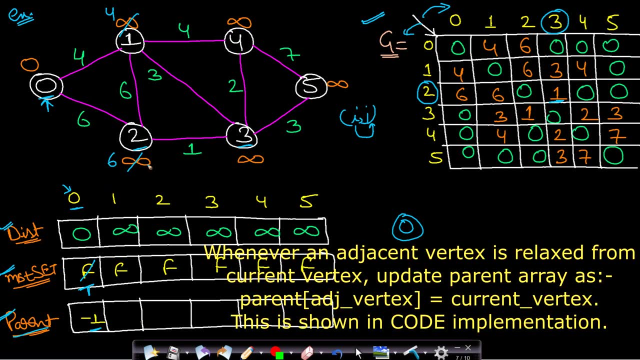 value infinity, and the new value which is proposed is having value four, since the edge weight from zero to one is four. so we will take minimum of four, comma infinity, which will be four. So it will be replaced with four And similarly, this will be replaced with value six. okay, now, this is basically maintained. 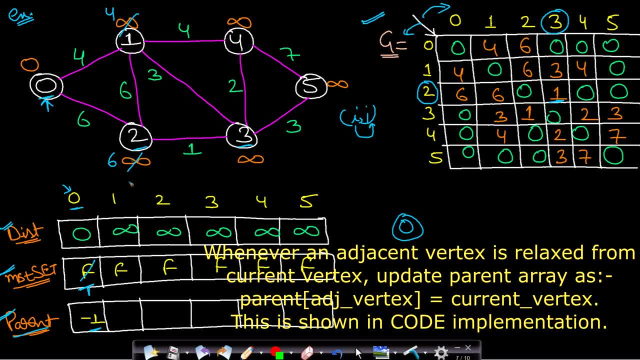 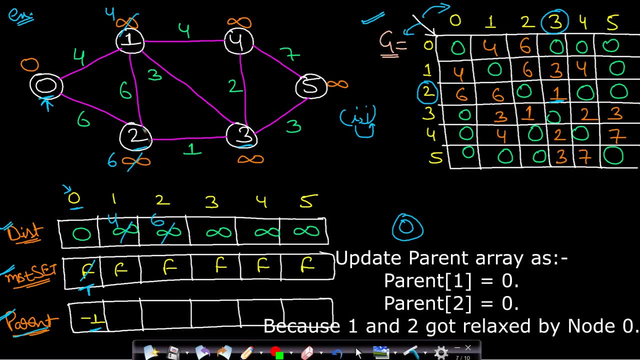 in this distance vector. so for this one it will come out to be four, and for this two it will come out to be six. I hope you are understanding how we are updating now. once this is done. so we will now go to the first step and we will select the minimum value. 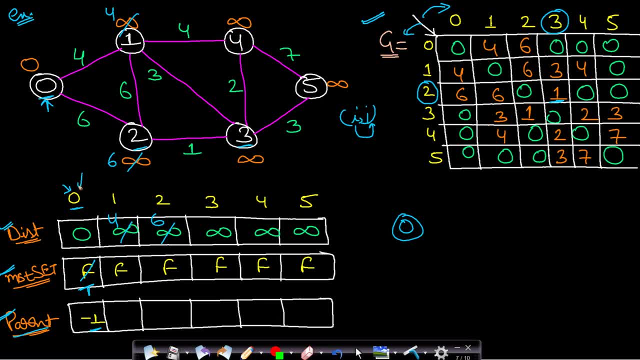 node. so we will start scanning from this node zero. So we can see that node zero is having value zero. but this is already included in MST set because this value is true here. Okay, So when MST set corresponding values true, we will just ignore this node. we will go to 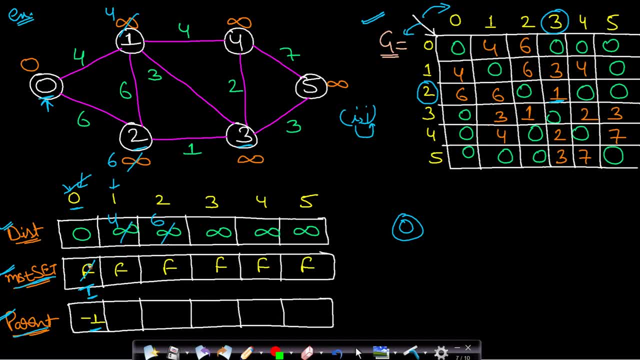 node one. now, node one, distance values four and MST set is false. This means this is not included, and so this is the candidate to get selected. So our candidate is one now and minimum value four, and if you keep scanning Then you will find that. 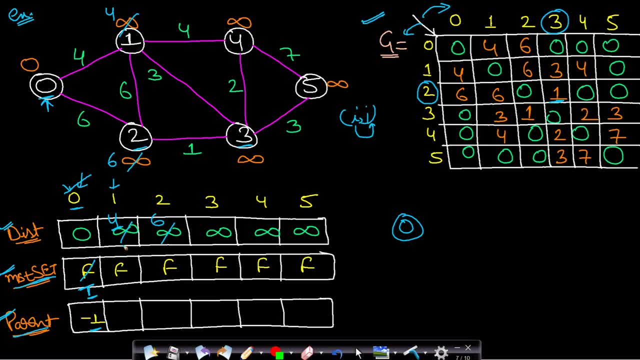 minimum value. so we will be including this node one. so we will make this first true. this is our second step, and in the third step, what we will do is we will relax all the outgoing edges. so let me just include this one. okay, we will now relax the outgoing edges. so from one the outgoing edges to 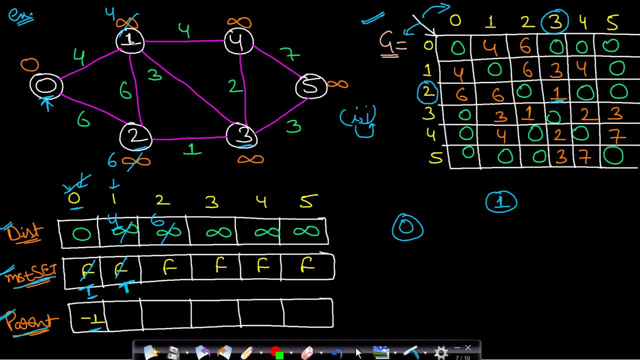 zero. but zero is already present in msd, set from one, outgoing edges to two, so from one to two that the weight is six, but it is already having value six. so it will not get updated because it will be picking the minimum of six comma six, which is six now from one and outgoing edge is going to three. 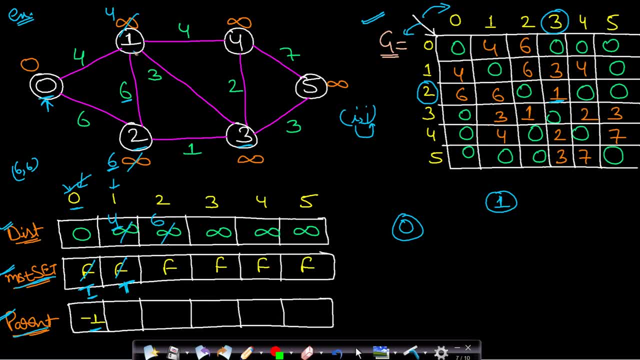 so this three is having value infinity and the new value proposed will be three. so it will take minimum of three comma infinity. so this will be three. so this three will get updated with value three. now from one we can go to four. four is having value infinity, so this will be updated. 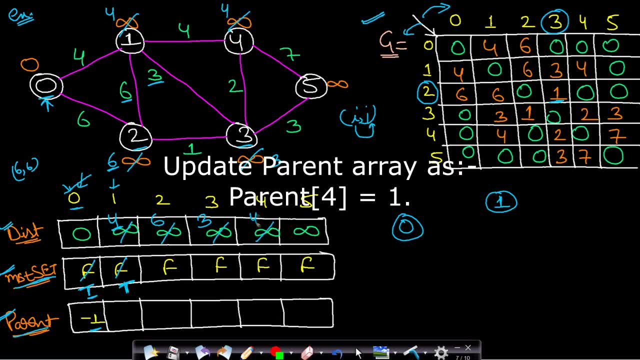 to new edge weight, which will be four. so four will be updated with value four. okay, and now this third step is also done, and from this zero to one, actually this weight is four. now this is our mst structure, this is the forming mst structure. now this node one has been processed. so once a node. 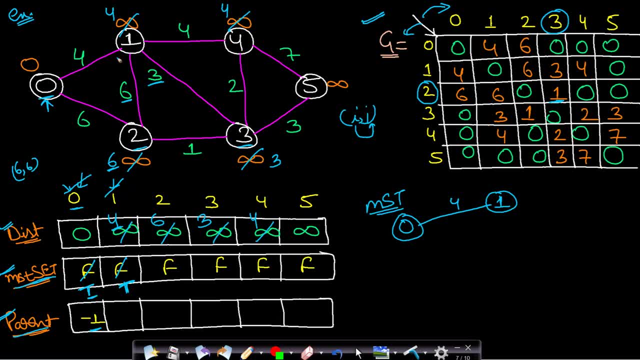 has been processed, then we will store its parent value. so what is the parent value of one? one's parent value is zero, so we will be storing value zero here, since from zero we reach to one. okay, now what will be the next node which will be picked? we will be scanning all these node values. 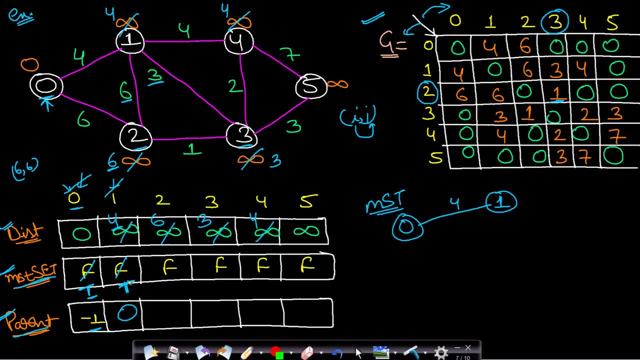 and zero and one are already included in this mst set, so they will not be the candidates in order to get selected, so we will start from this two. so two is having value falls. this is not present in mst set and the distance value is six for three, distance values three. so this is the minimum. 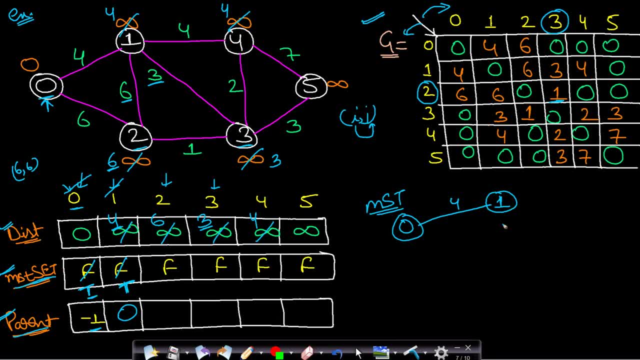 value. if you keep scanning, you will find that three is the minimum value, so next candidate is three. now from what node we jump to this three? we jumped from node one to node three, so the parent of node three will be node one. okay, now, since three has been selected, it is having 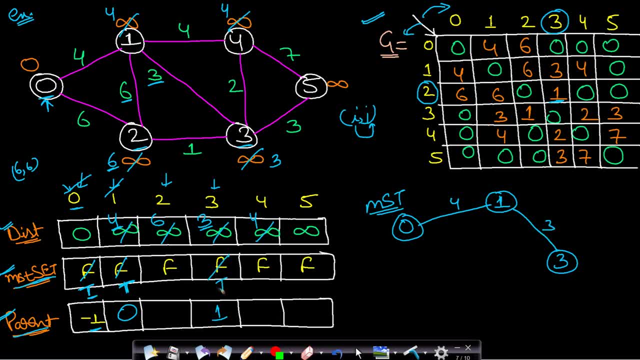 edge, weight three. so the next step is to make it true, since it will be included in the mst set, and then we will be relaxing all the outgoing edges. so from three- there is one outgoing edge- to two, and the value at two is already stored is six. but 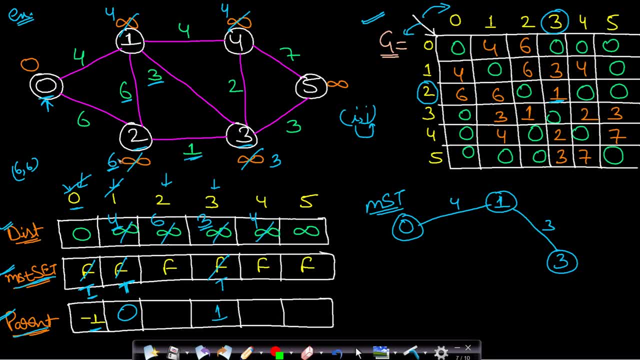 three to two, the value is one, so we will pick minimum of one comma six and this will come out to be one. okay, now what will happen at the next step? at the next step we will see. from three to one, there is an edge, but one has already been included, so nothing will be done. it is included in the mst. 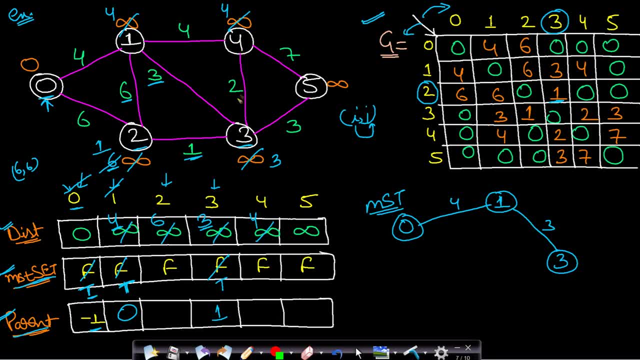 set from three to four. there is an edge from three to four. uh, the distance is two and at four the value stored is four. so we will pick the minimum of two comma four, which will be equals to and from three to five. we have distance equals to three. already stored value at five is Infinity, and 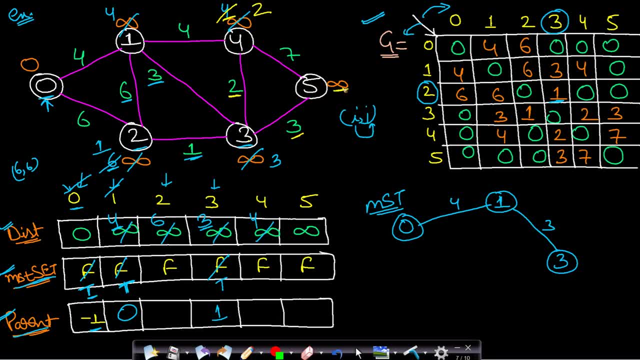 so the value which will get stored at five will be minimum of three, comma Infinity which will be equals to three. so this infinity will now be gone. so what will be the value updates? from three to two, value has now become one, so this will become one. from three to four, value has become two. 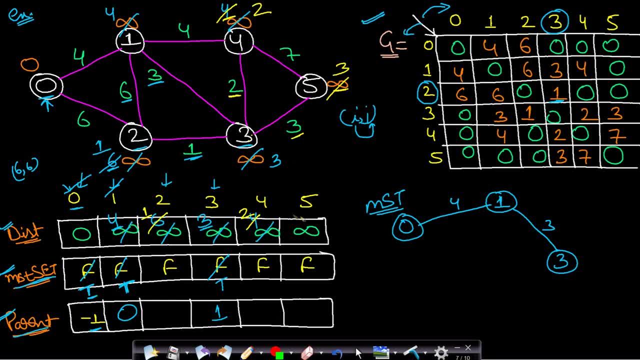 and from three to five the value has become three, so this will now become three. I hope you can see now, once you have updated all these values, so all your steps are now done. now you will again move to the first step. so you have processed 0, 1 and 3 and you have marked them as true. they are. 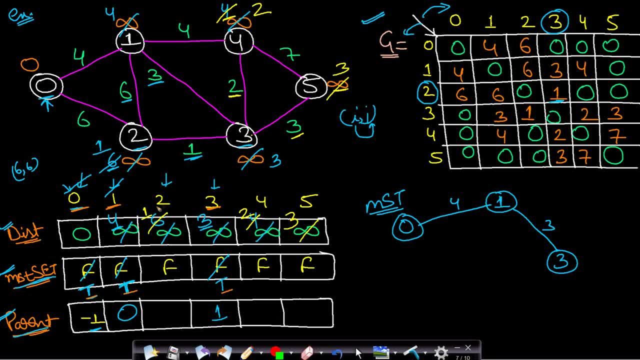 included in mst set. now for the next part. only three nodes are left: 2, 4 and 5. so you will pick the minimum value. minimum value is for 2, so this 2 will get selected now you will make this value true and you will also store the parent. so this 2 got a call from this 3. so 3 is the parent of 2. 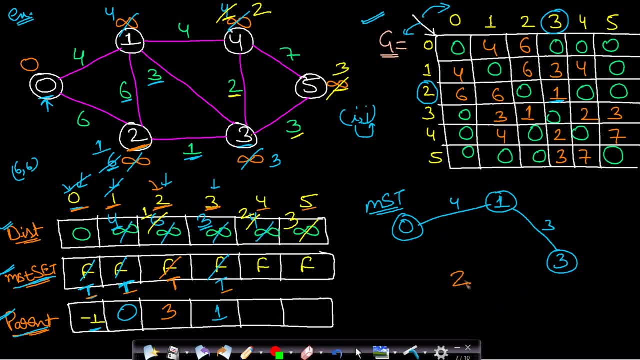 okay, and now 2 will also get selected, so you will include 2 and this is having edge wet 1. now all the outgoing edges from 2 will be relaxed, but you can see that 0, 1 and 3 are already included in mst. 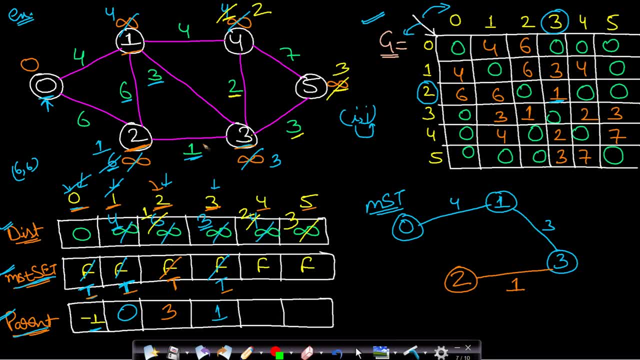 set, so nothing will be done and you will move back from 2 now. all these three steps are now done and 0, 1, 2, 3 have now been completed, so you can see that 0, 1 and 3 are already included in mst set. so 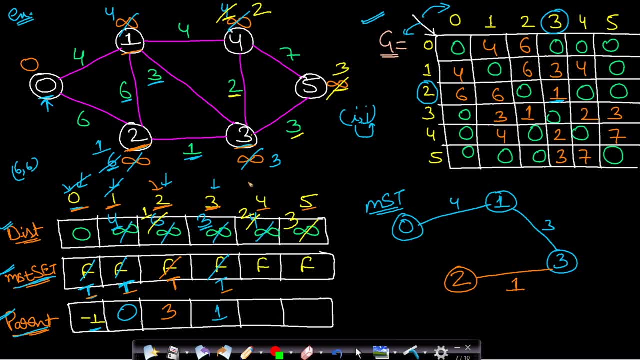 we will again go back to step 1. step 1 was to select the minimum value node. so the minimum value node, that is, the node with the minimum weight among 4 and 5, is 4, which is having value 2. okay, so this 4 will get selected. so this is node 4 and the edge weight is 2. so once you select this, 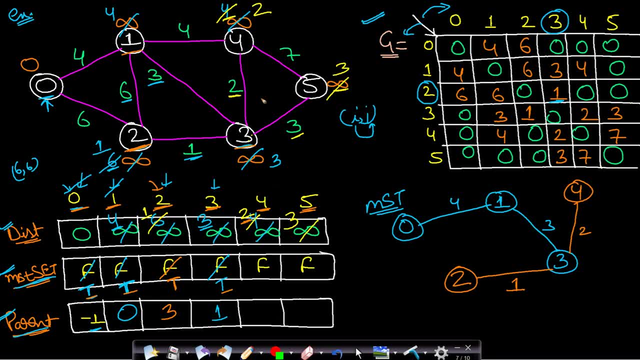 4, then you will have to store the parent. so the parent for 4 is actually 3, okay, so you will have to store the parent. for 4 and 5 is actually 3, okay, so this is node 4 and the edge weight is 2. so 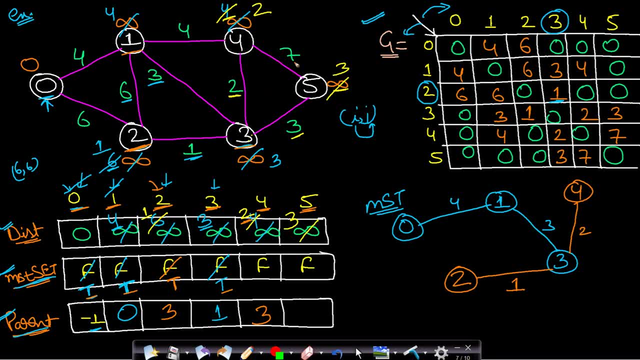 you will also be relaxing all the adjacent edges. before relaxing, you will be making this mst set at 4 true, since you have processed this, that means included this node, and after that you will be relaxing the adjacent edges. so 1, 3 are already included and 5 is not included. and the distance 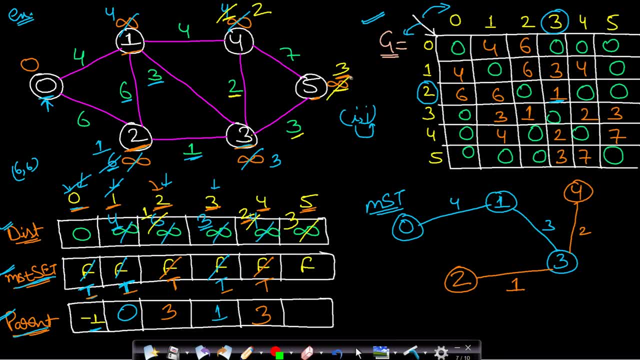 from 4 to 5 is actually 7, but already stored value is 3, so nothing will be done. so we have processed this node 4, so this is already included. so we have processed this node 4, so this is already also done. and now, again, we will go back to step one, which is to select the minimum value node. 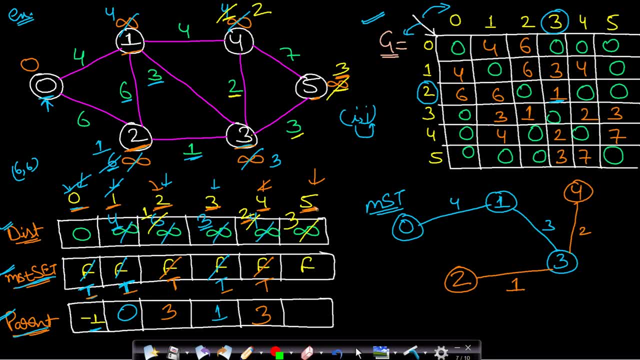 that is the node with the minimum weight. so we are left with only one node, which is five, having value three. so this will obviously get selected and the edge weight is actually three, so this is three and the parent node is actually three and this will become true. so these are the steps. 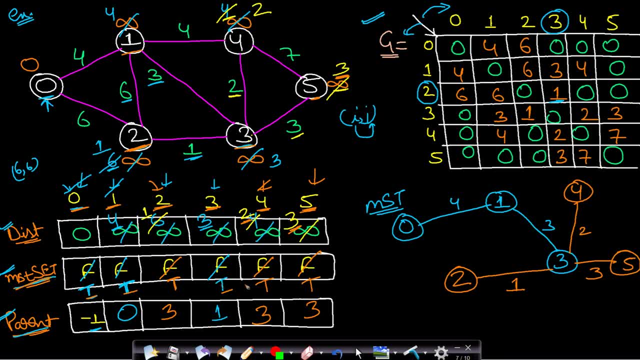 now you can see that all the vertices are true, are marked true because all the vertices have now been covered in our graph and whatever structure is formed is our minimum spanning tree and this structure is basically represented by using this parent array. now, throughout the explanation, i found the edge weight from this graph, but actually in the code you will be. 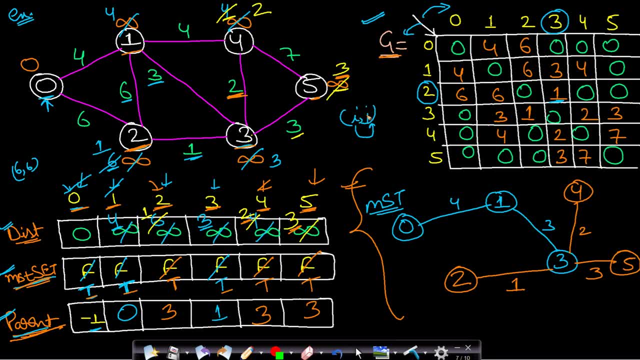 finding it by using this adjacency matrix. if you have i comma j, then your edge will be going from i to j, and the edge weight can be found by going to ith row and jth column. whatever value is stored, that is the edge weight. okay, so this is it about the brems algorithm. now, by using this parent, you can. 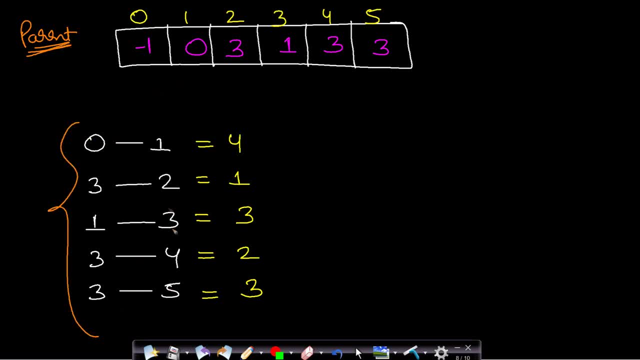 actually print your structure. so this is how you can print your structure: from 0 to 1. your value is 4. you will actually start iterating from this node 1, because for node 0 there is no parent. so there will be some other node which will be pointing to this node 0, because the entire graph 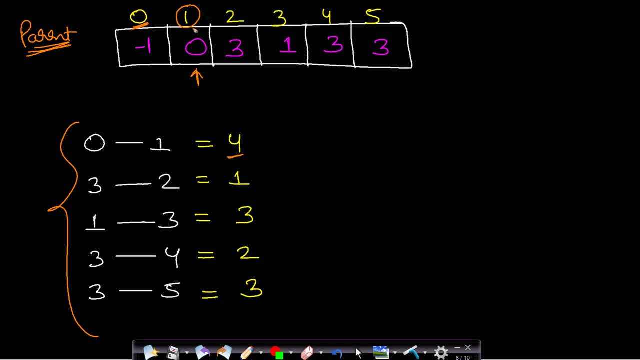 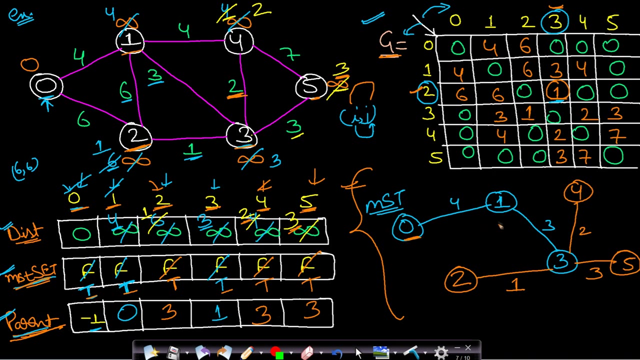 is connected. okay, so we will actually be starting from this node 1. we will first print the value and then we will print this index. you can do it in the other order as well, so I will first print the value. from 0 to 1: the weight is 4. you can see that in the graph as well. from 0 to 1, the weight is 4. 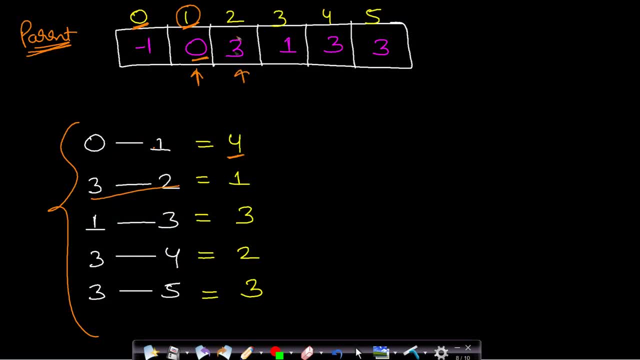 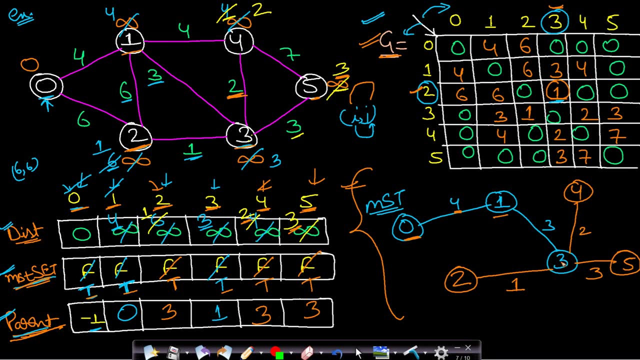 now we will be printing from 3 to 2. the weight is 1. this weight can be printed by using this graph. that is, this adjacency matrix. now, from 3 to 2, the edge is 1. now it is not important to print all these values adjacently. 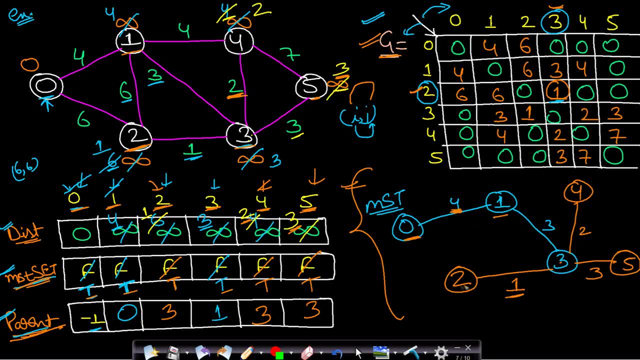 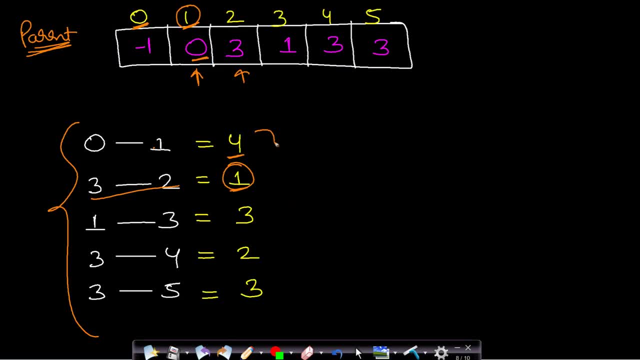 you can print: from 0 to 1- weight is 4. from 3 to 2, weight is 1. from 5 to 3, the weight is 3 and something like that. okay, so it is not actually important to print it adjacently, but this is. 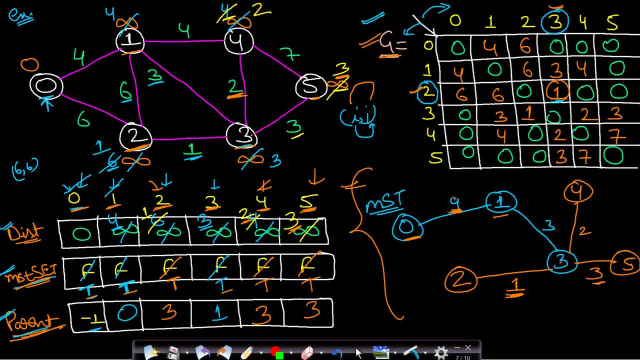 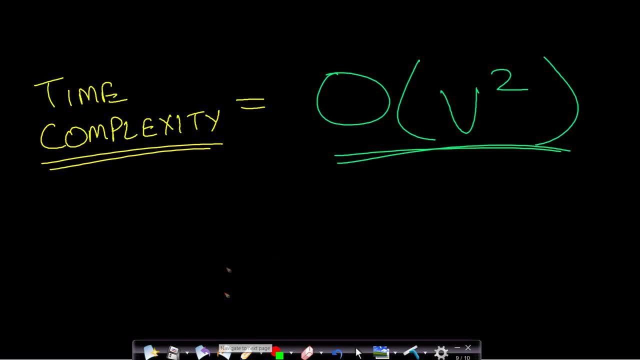 showing the structure. by using this knowledge you can form the MST, this structure. okay, so i hope you understood the intuition behind coding this entire prims algorithm. now the time complexity for this will be order of v square and i will be explaining this in the code. this will be very 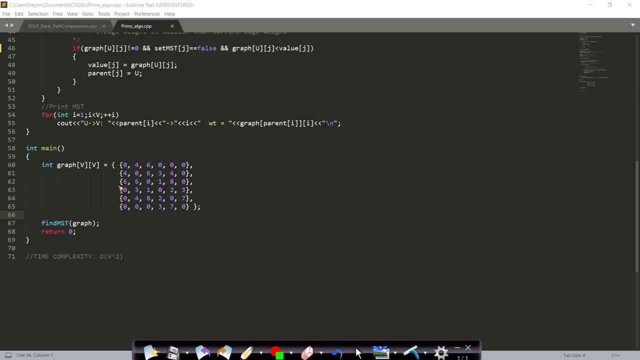 simple from the code. so let us now look at the code. this is a simple code for the prims algorithm. now, in this case, i have taken v, value equals to 6, where v is the number of vertices. this is the graph. you can see that i have taken v, value equals to 6, where v is the number of vertices. this is the graph. 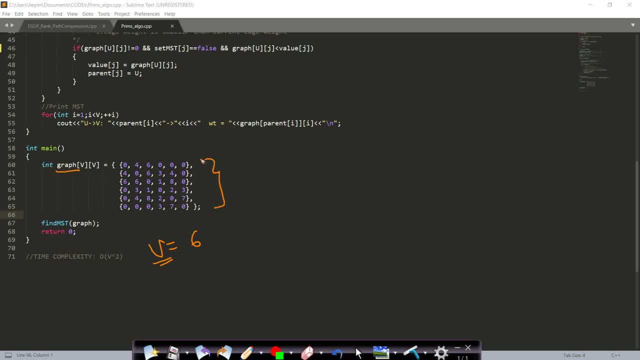 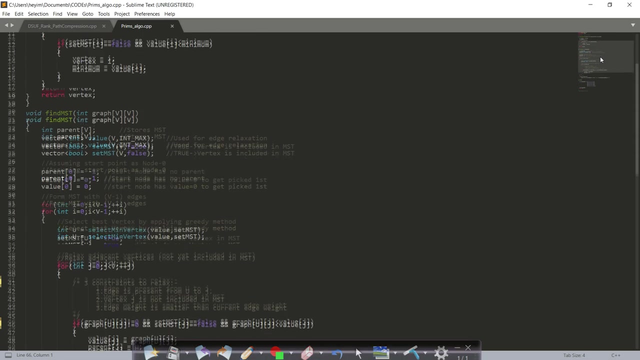 where v is the number of vertices. this is the graph. this i have manually formed, okay, and this is nothing but the adjacency matrix, so i hope you understood this now. once we have formed the graph, then we can use the find mst function in order to find the minimum spanning tree. so let us now look at the minimum spanning tree here now. this is the. 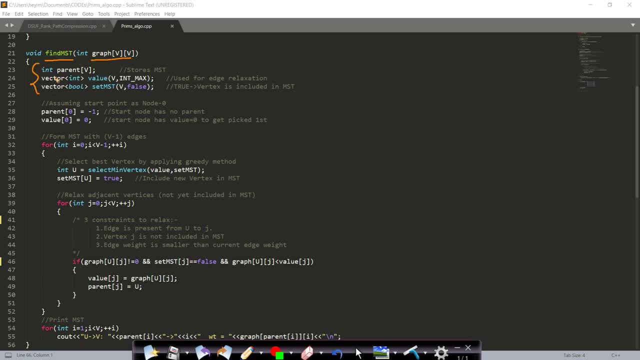 find mst function. we will be receiving the graph and we will be taking all these three arrays, as i have explained you, according to the requirement. the first one will be for storing the mst structure, which will be the parent array. the second one will be for edge relaxation part, so it will be. 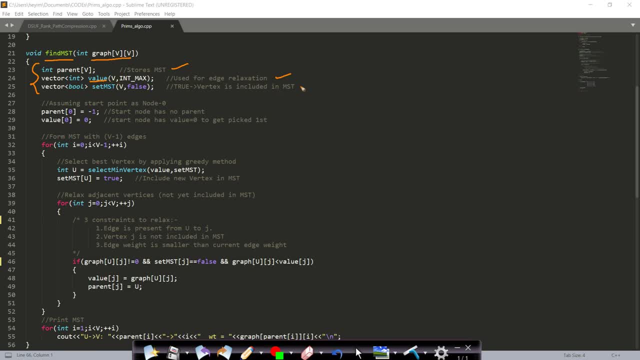 storing the a, the node values, and the third one will be storing the set mst, that is, the nodes or the vertices which are already included in the mst. okay, and after that we will start our algorithm. so i have assumed that i will be starting from source. node equals to zero, so in this case, 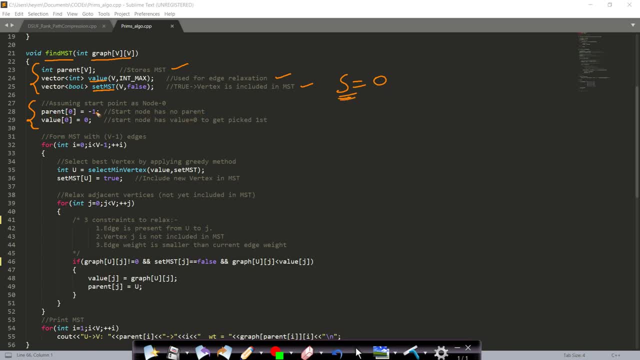 for the source node there will be no parent. so parent at zero will be equals to minus one and value at zero will be zero. because for the source node i already showed you that the value, that is, the node weight value, will be zero, so that it gets picked first because our algorithms first step is to scan. 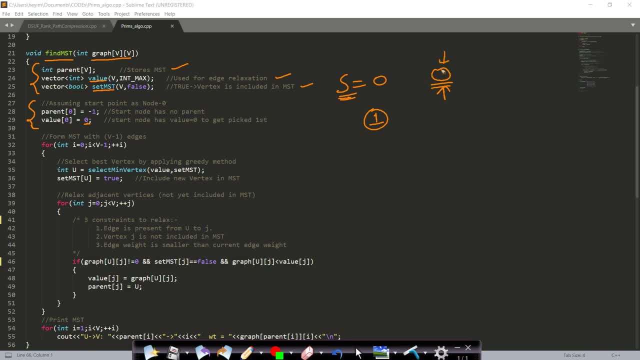 through all the vertices and then find the vertex with having the minimum node weight. okay, so we will assign initially the source node with value zero and all the other nodes with value infinity. so this is the logic for assigning value at zero equals to zero. now, once you are done with all the 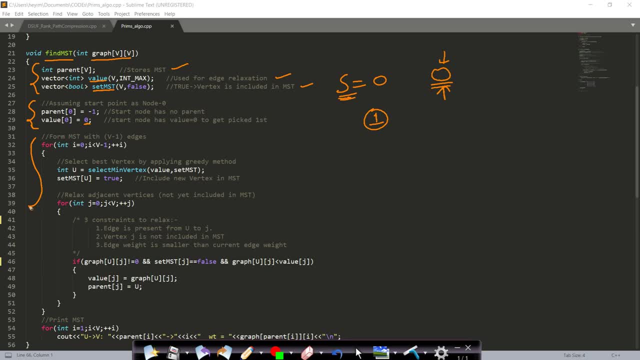 assignment part. so we will follow the algorithm, and this is the mst algorithm, the main algorithm. okay, now here. we already know that this is a connected graph, this has to be a connected graph and it will be having, let's say, v number of vertices. then it will be having v minus one. 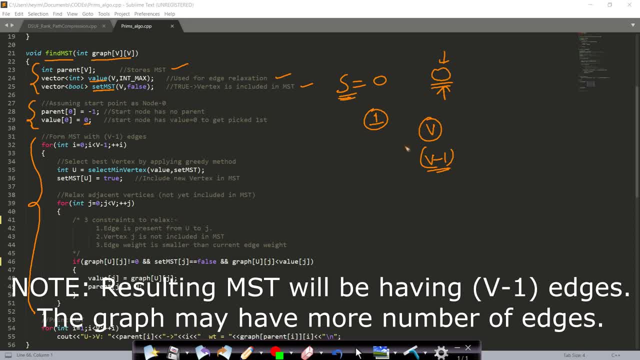 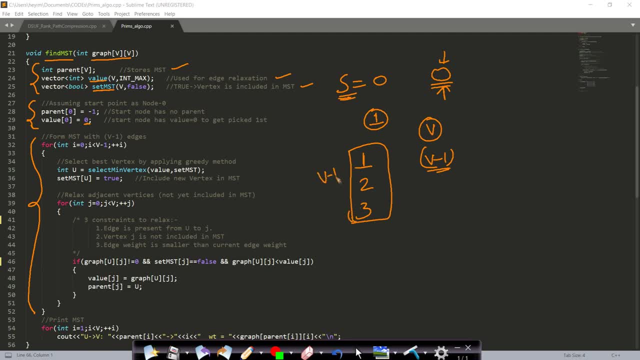 number of edges. so how many times do we need to process this algorithm? that is step one, two and three. as i have explained you in the theory, we will be repeating these steps v minus one number of times. okay, so the outer loop is for defining how many times we will be running all these three steps. 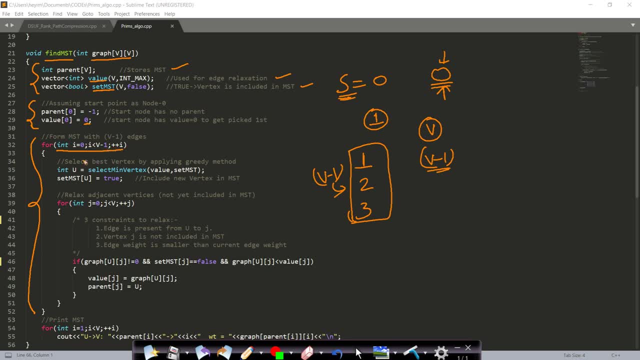 we will be running it v minus one number of times, so inside that we will be following each and every step one by one. so this is nothing but step one. so step one is for selecting the minimum node: weight, that is, the node having the minimum weight and that will be stored in u? u is nothing but the. 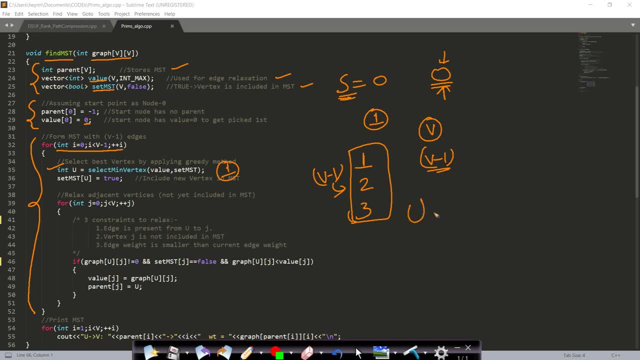 starting node. so our edge will be going from u to j. okay, so this will be something like: uh, you will be selecting u and then you will be finding what is the appropriate j. so first we have found the node having minimum weight, which is stored in u, and now we will be making the set mst at u. 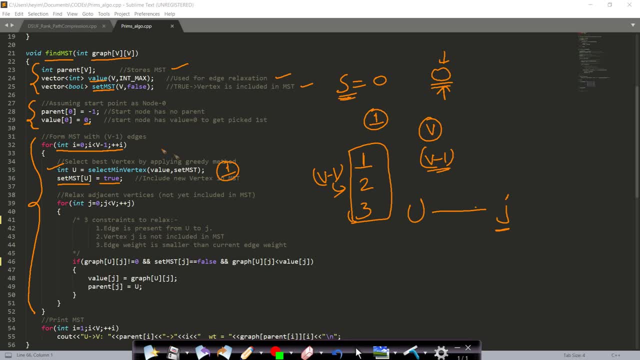 equals to true, since u will now be assumed to have included in our mst set now step one, and this is step two. step one and step two are now done, so this is nothing but step three. now for this step three. what we will do is we will relax. 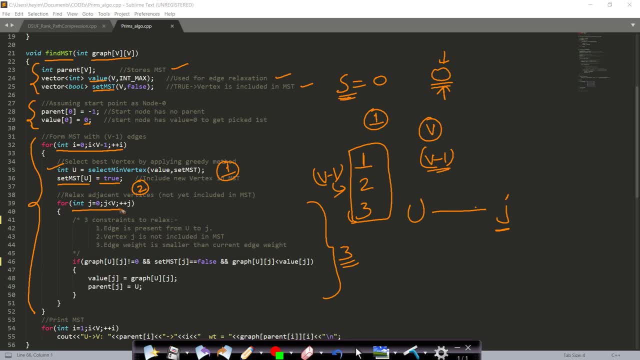 all the adjacent vertices. so we will scan through all the vertices in order to find which are the adjacent vertices. so in this case we have three constraints. that is, uh. the first constraint is that if you are using the mst set, then you will be using the mst set and you will. 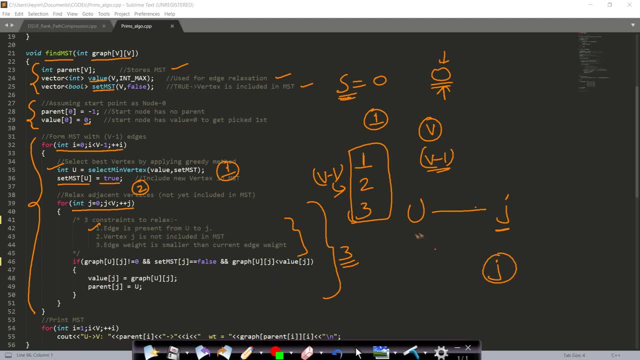 have to sorry, let me, let me just select the mst set with rotation. so this is your corner. videos will not work for that. so next step: once this is completed, uh, the next step. you will have a problem with over doom. the most common over doom is that, uh, if you are using the mst set, 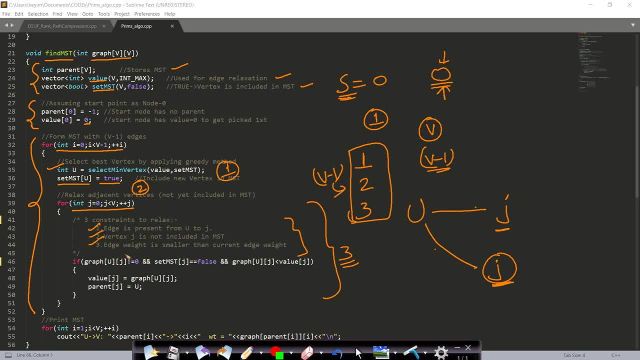 where we have already alreadyılan mst sete and when we also actually have a node accepts, we are going to use somenode. so this one, of course, will be much easier to in whatever scenario or anybody might alreadywant to use modern j, so we will start with modernカ. now it's pretty easy to understand. it's just an example, because you can write down whatever the type of node is you want. so if i put log точ, can any membrane or I will also. for example, few modules can be used for texting you multiple times, so this command can be used in determinations. 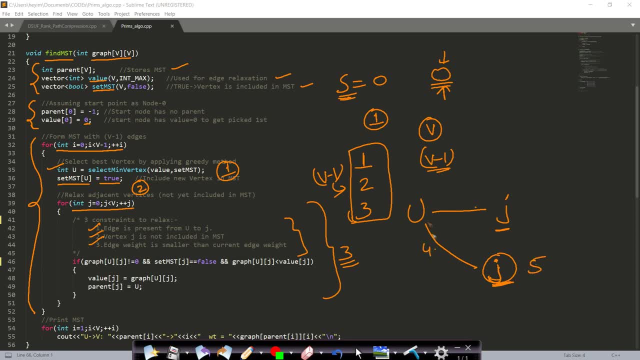 instead you can reply to this command. so, according to most important things and this command value- let's say it is having value 5 and this edge is having value 4- then since this is having value 4, then minimum of 4 comma 5 will be 4 and so this will become 4. so only in this condition, if first. 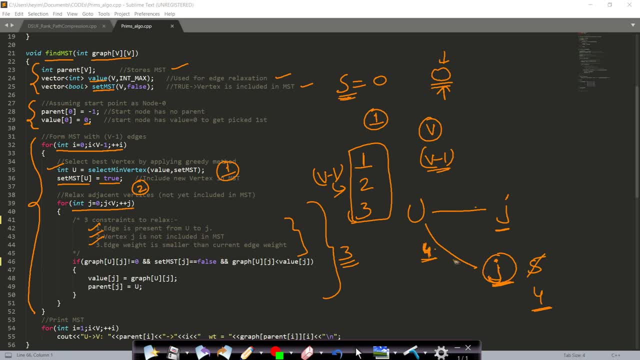 two conditions satisfies, then we will see if the edge weight is lower than the already stored value. only then this node j will get relaxed. okay, so these are the three requirements. therefore, the first requirement is that there should be an edge from u to j, so the edge value should not be zero. 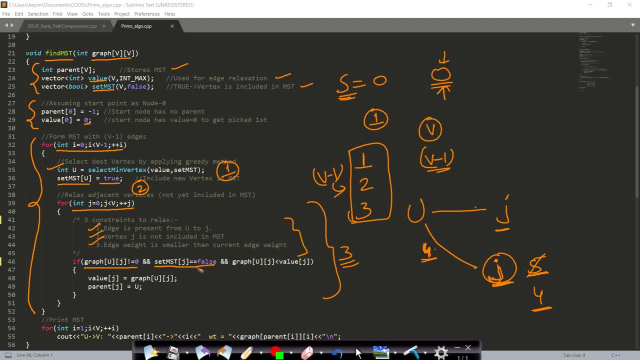 now. the second requirement is that the node j should not have been included in the mst set, so it should be false. and the third requirement is that the current edge value, which is graph, at u to j, that means this edge should have less value than the already stored value at j, which is value at j. 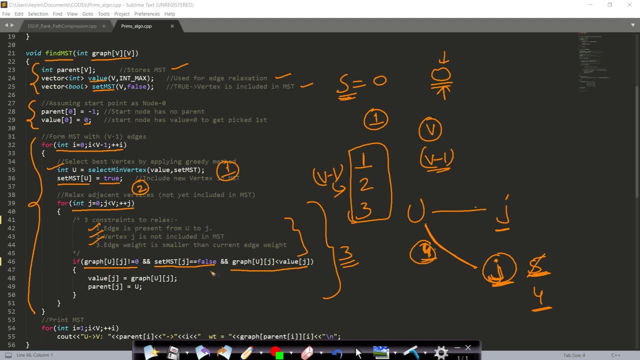 okay, now, if these three conditions satisfies, then only we will relax that node. so we will store the new value, that is, value at j will be equals to graph at u, j, which is nothing but 4 in this case, and after that we will also be updating the parent at j, so the parent at j 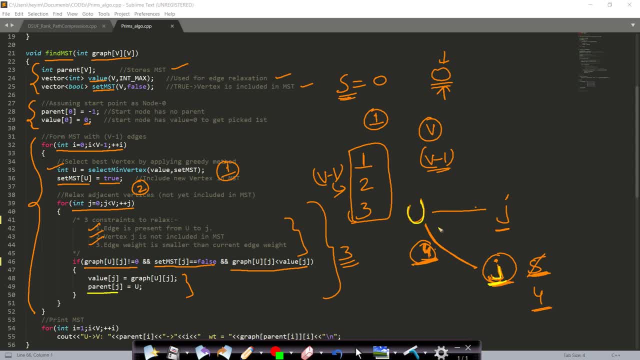 in this case, will be equals to u. okay, so this is how we are updating the parent. so once we have relaxed a node, then the parent will get updated. so in this case, the parent will now become u. so these are the three steps and these will keep repeating: v minus 1 number. 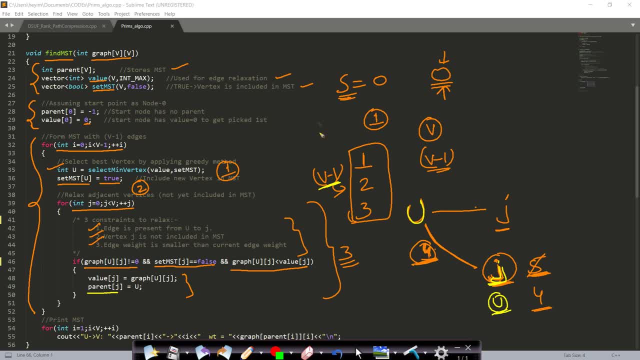 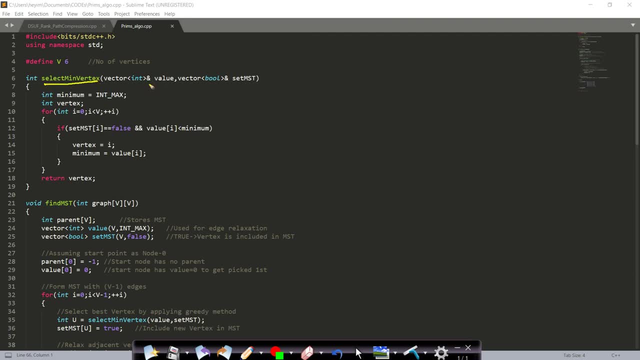 of times, unless we have included all the vertices in our mst. so let us now look at this select min vertex function. now, this is a select min vertex function. here we will be taking the value and we will be taking the set mst. so value is nothing but storing all the node values, that is. 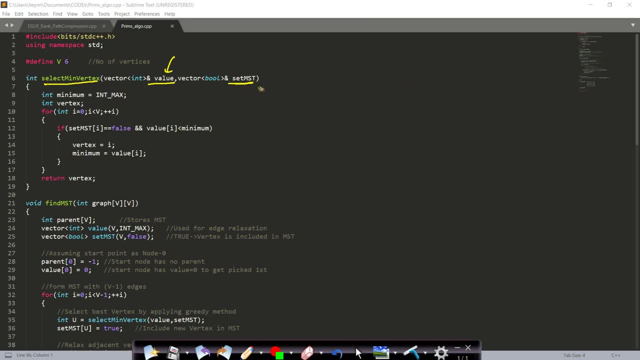 all the node weights, and this set mst is keeping track of all the nodes which are already included in mst. so now what we will do is we will only scan through all the nodes that we have stored in the set mst and we will see if the current node is not included in the mst and the current node value.